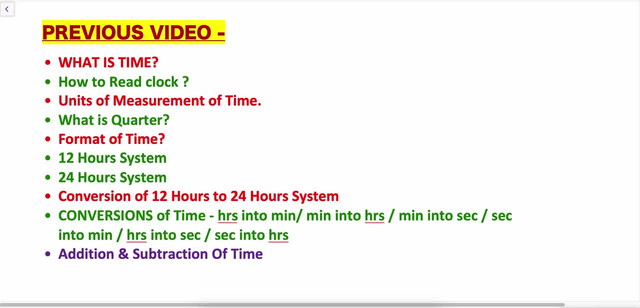 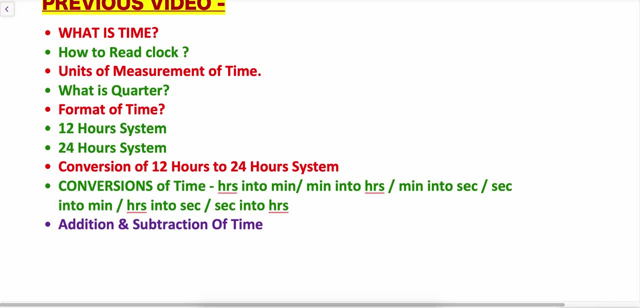 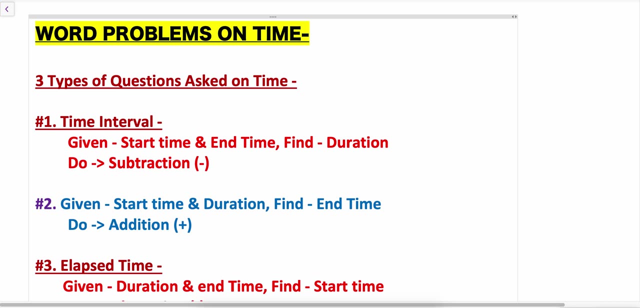 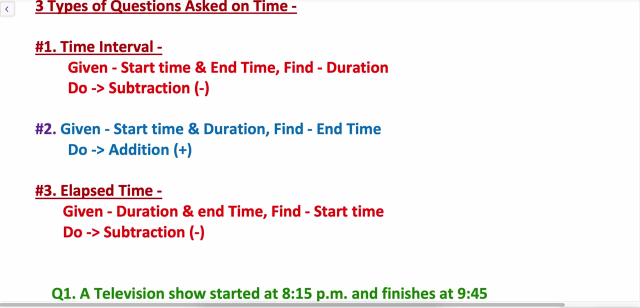 So do watch my previous two videos On time to get the detailed knowledge of the units of measurement of time and the conversions and also the addition and subtraction of time. Now let's begin the today's video. Today's video is all about the word problem, word problems on time. So in exams three type of questions are asked on time. First question is asked on the time interval in which the given, the given information will be the start time. 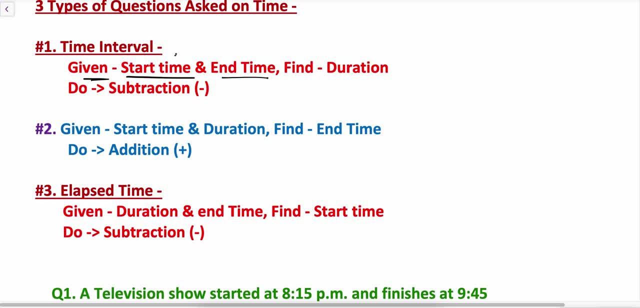 And the end time. So in some questions the start time is mentioned and the end time is mentioned and we need to find the duration, duration or the time interval that how long the the movie last, or how long the the meeting held, something like that. So for that to find the time duration, we need to subtract, we need to subtract, we need to do subtraction: end time minus the start time. 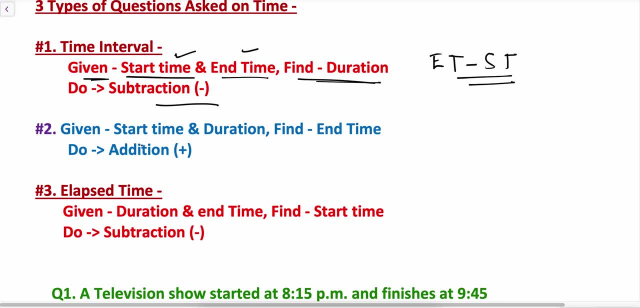 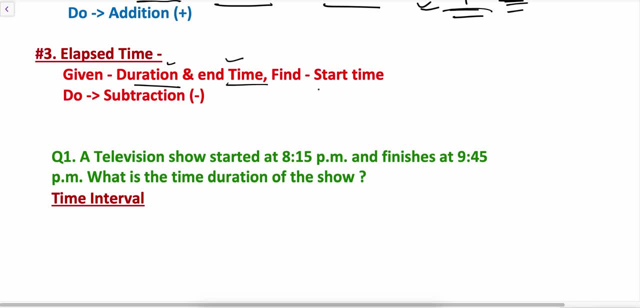 and the end time is mentioned, but they will ask the start time. so to get the start time, if this is the end time and this was the duration and we need to get the start time, so to get that start time we need to go backward and for backward 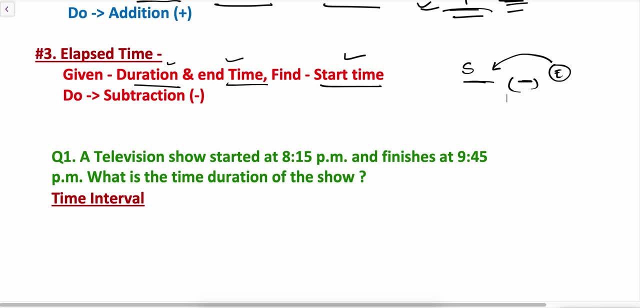 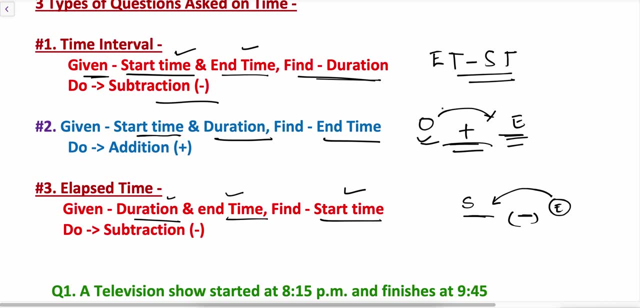 we need to subtract. but to get the, to get the start, to get the end time from the start time, we will move forward. so we need to add here, but to get the lapse time or get the start time, we need to go backwards. So for that case we need to. 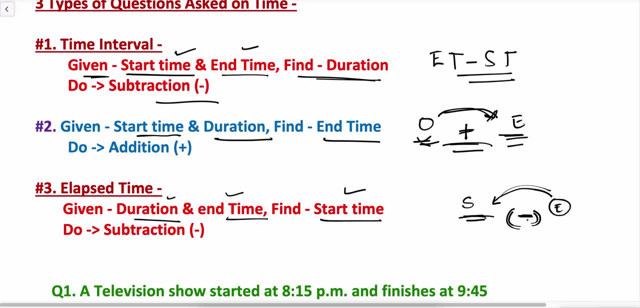 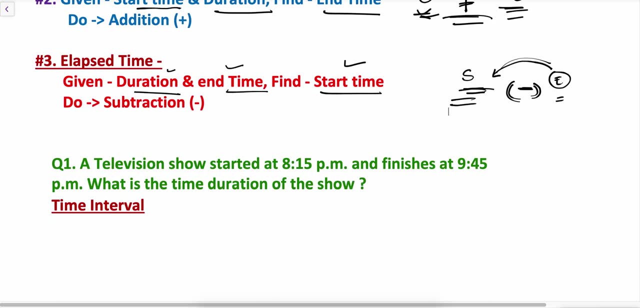 subtract here, Subtract the duration from the end time to get the start course start time. so this is. these are the three varieties of question asked. I hope the concept is clear to you now you will not get confused how to solve the problems on time. so let's see some examples on that question one: a TV show. 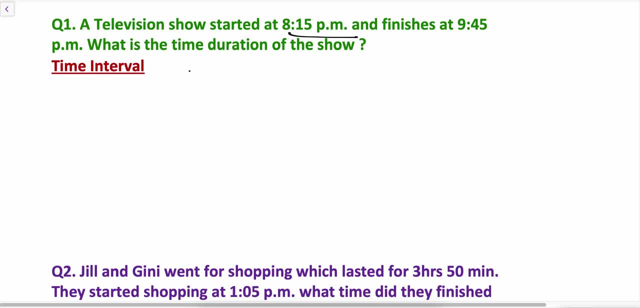 started at 8: 15 pm. so here the start time is mentioned and finished at 9: 45 pm and time is also mentioned. what is the time duration of the show. so here they were asking the time interval, time duration. so to find the duration, what we 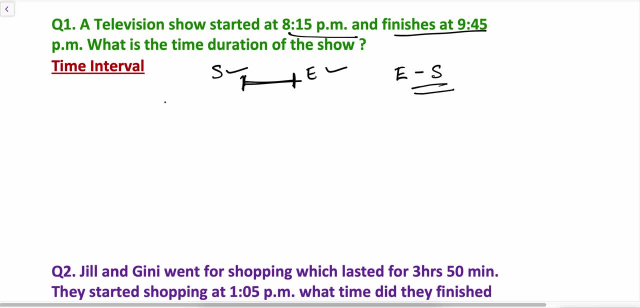 will do end time minus the start time here. so what is the end time? 9, 45 this is our and this is minute. 9, 45 minus 8, 15, so 5, and we will start from the left hand side. so 5 minus 5, 0, 4 minus 1 is 3. 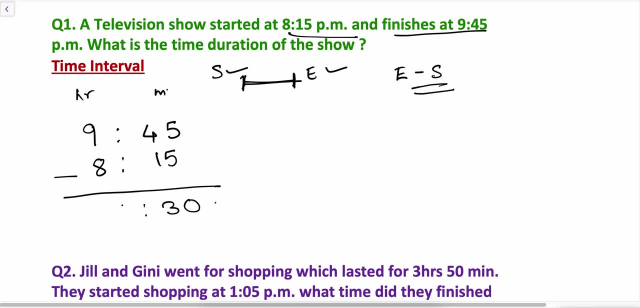 3, 9 minus 1, 8 is 1, so the duration of the show was one hour 30 minutes. one hour 30 minute. so this is how we can find the duration when the start time is given and when the setup is motion and the end. 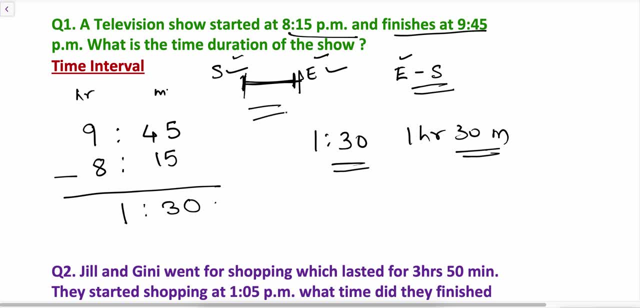 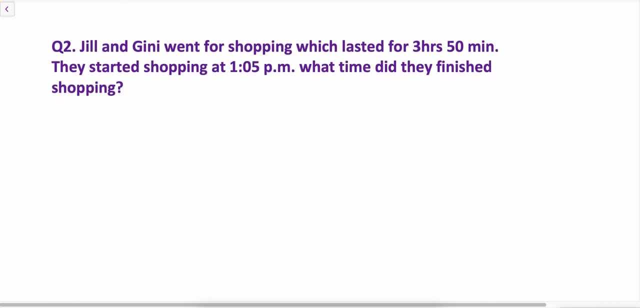 dimensions and we need to find the duration. so what we will do? subtract the strata from the end time to give them time interval. now let's see another type of question. jill and guinea went to, went for shopping which lasts for 3 hours 50 minutes. so here duration is given and they started shopping at 1, 5 pm. 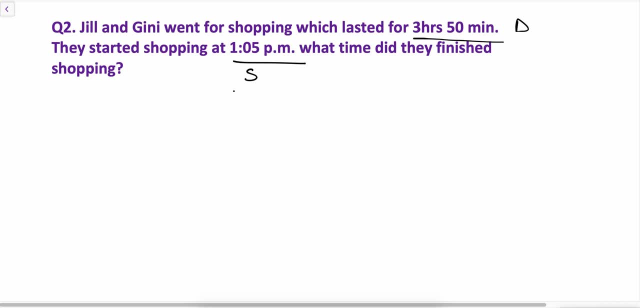 and this is the start time. what time did they finish? finish the shopping? so end time. we need to find. so, when the start time is mentioned, and we need to, and the duration is mentioned, and we need to find the end time, we are going forward, so we need to add, so add the start time and the duration. 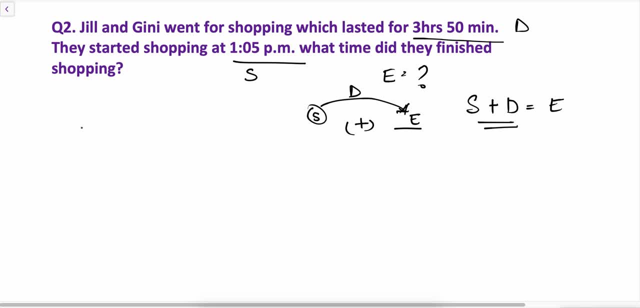 to get the end time. so what's the start time? here one five, this is hours, and this is minute. one, five as a starting time, and the shopping goes for three hours, 50 minutes. add them, so five plus zero five, and here also five, and this is four. so what time did they finish the shopping? it is 4, 55. 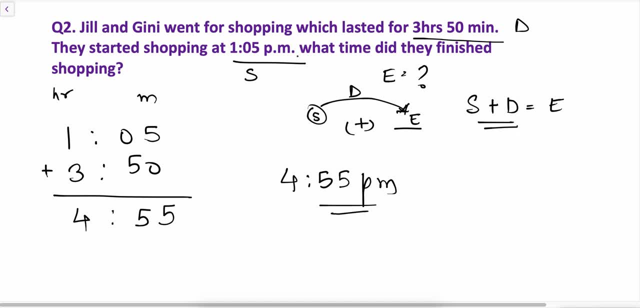 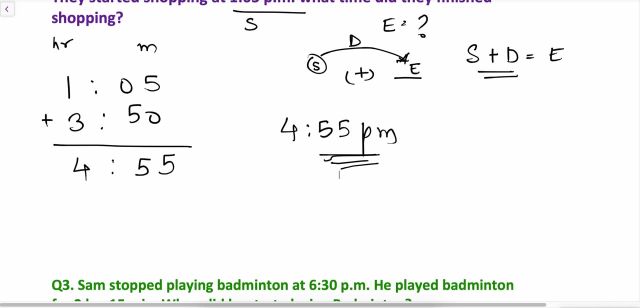 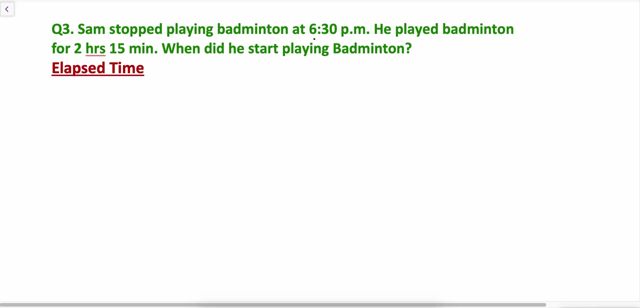 pm and they started at 1: 5 pm and the end ended shopping at 4: 55 pm. so this is how we can find the end time. now let's see one more type of question. sam stopped playing badminton at 6: 30 pm, so this is the end time he stopped playing badminton. 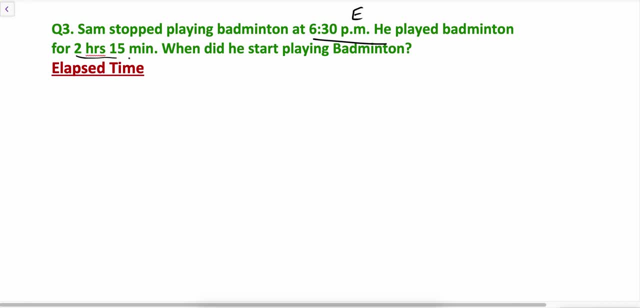 he played badminton for 2 hours 15 minutes, so this is the duration given here. when did he started playing badminton? so the start time we need to find here. so start time is not mentioned, but the duration is mentioned here and the end time. so when the end time is. 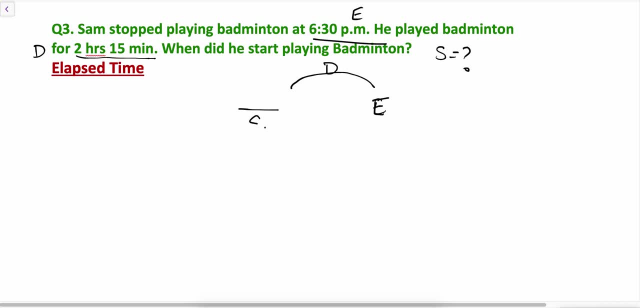 mentioned and the duration is mentioned. to find the starting time, we need to go backward. so what we will do, we will subtract. we will subtract duration from the end time. so end time minus duration will be the starting time. so let's do it. so the end time is 6: 30. 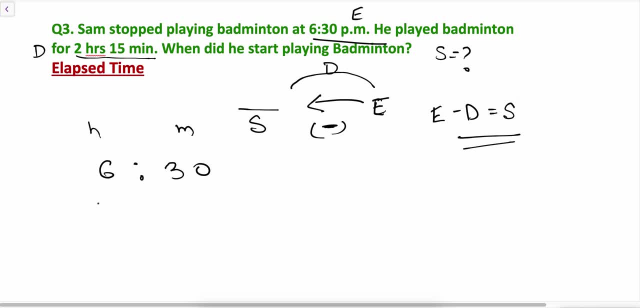 pm. this is hours and this is minute and the duration is 2 hours 15 minute. do the subtraction here: 0 minus 5 is not possible. we'll take borrow here, so it will become 10 and it will be 2.. 10 minus 5 is 5, 2 minus 1 is 1.. now 6 minus 2 is 4.. so the starting